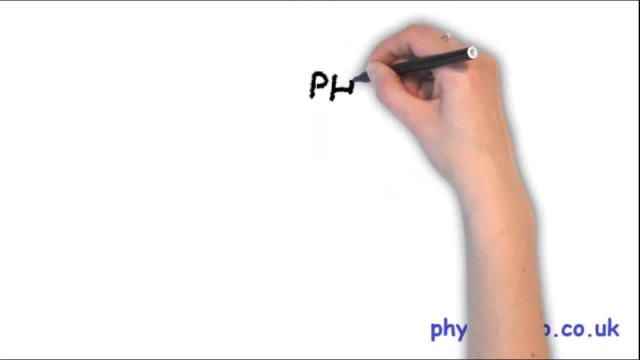 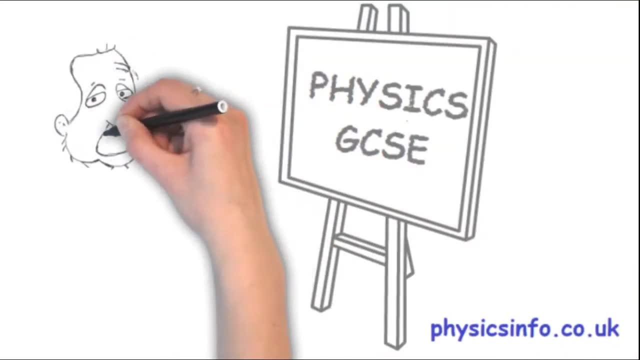 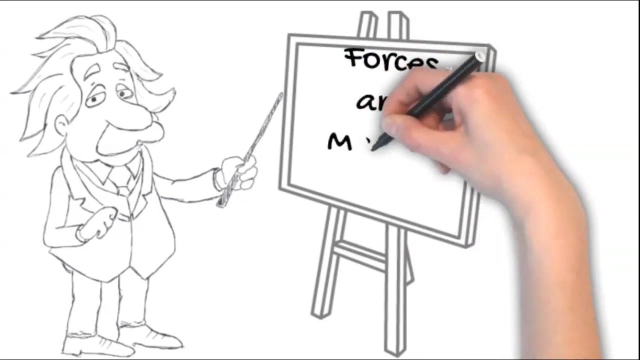 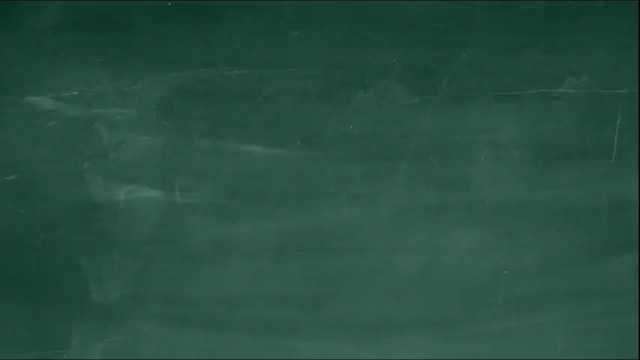 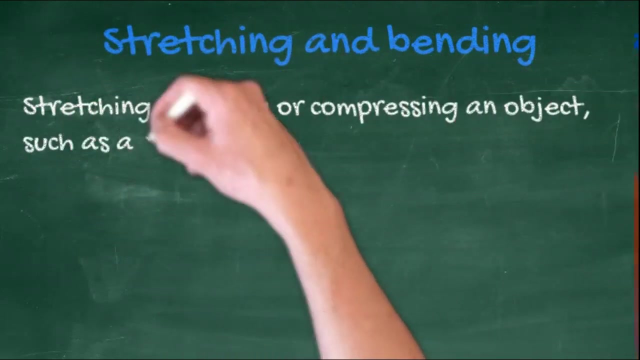 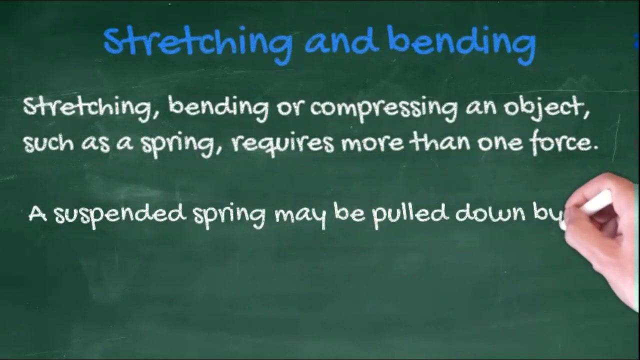 physicsinfocouk, Another in the series of Physics GCSE Tutorials, Topic 15. Forces and Matter- Separate Science. Stretching and Bending. Stretching, bending or compressing an object such as a spring requires more than one force. A suspended spring may be pulled down by a weight that's a force, but it is at the same time pulled up by the stand that's supporting it. 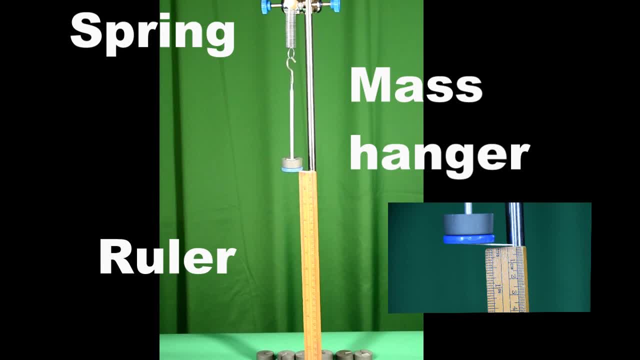 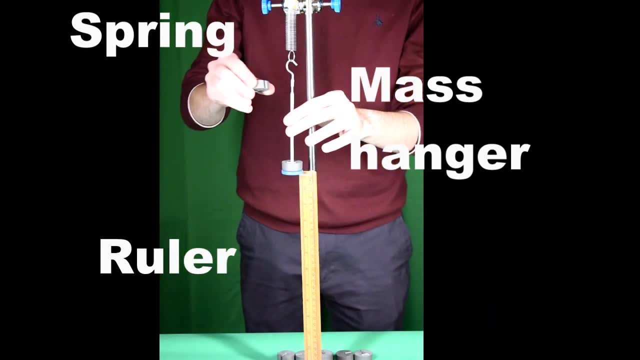 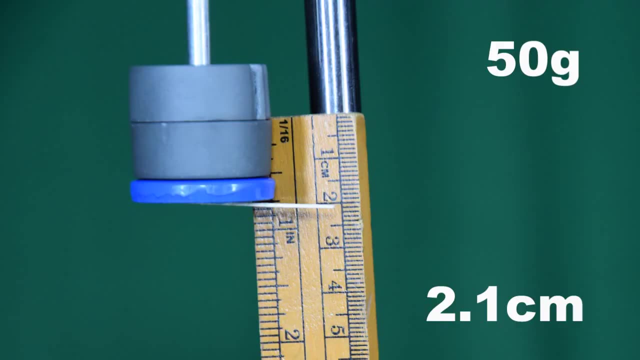 The spring is suspended from a clamp stand with a mass hanger hanging from the bottom. 50 gram mass has already been added. The hanger is set up at 0°, So 50 grams is now added and the extension recorded 2.1 cm. 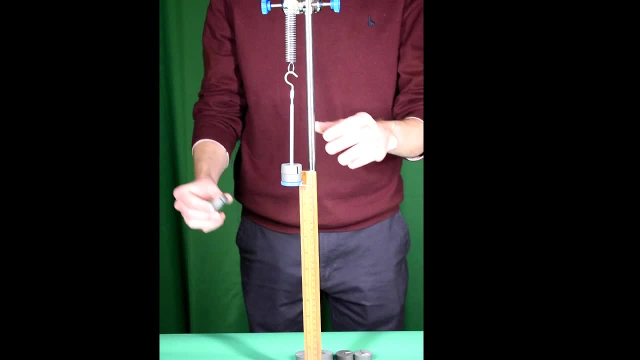 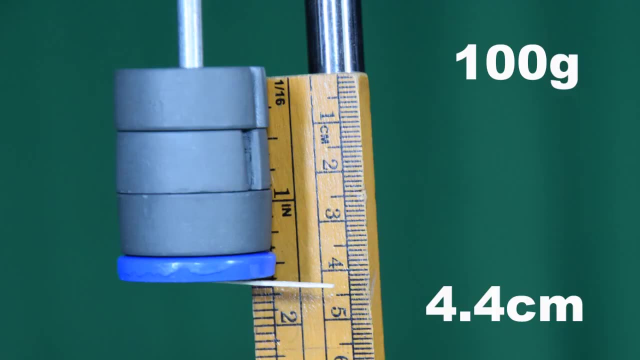 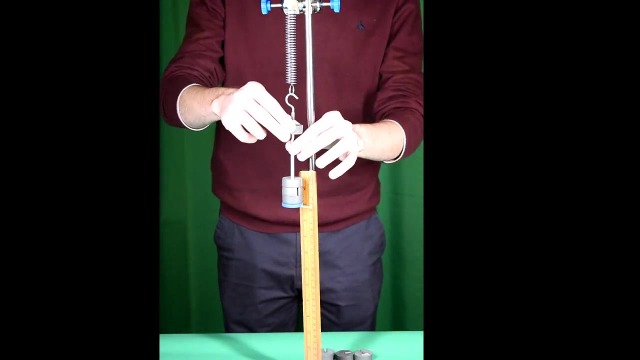 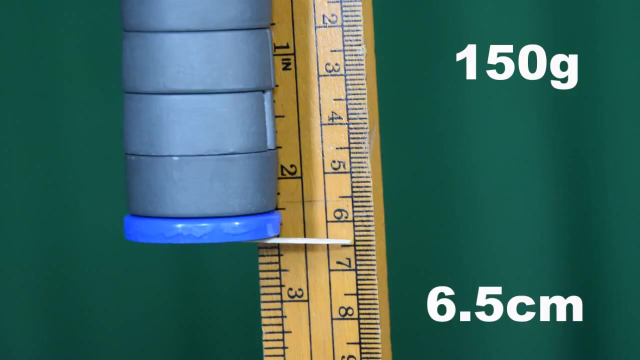 Another 50 grams is added. so that's two added masses and again the extension recorded, 4.4 cm, And another 50 grams. Note the use of the reference point at the bottom of the mass hanger: 6.5 cm. 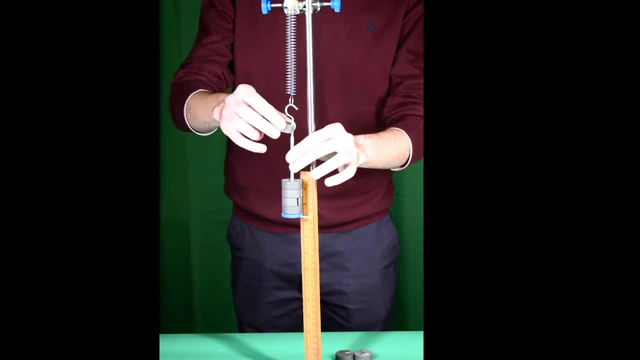 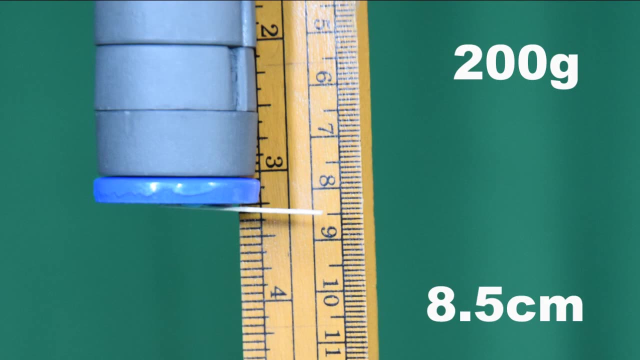 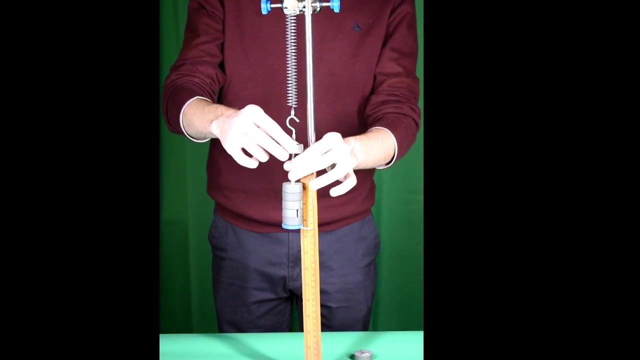 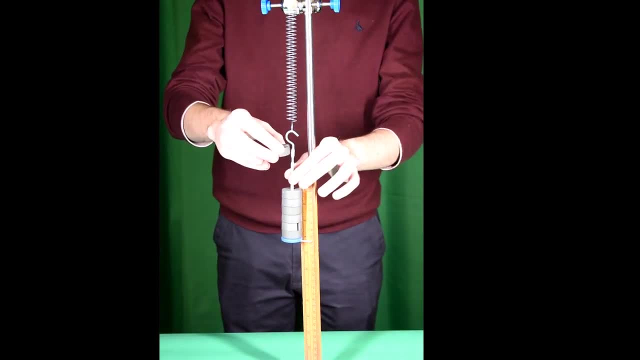 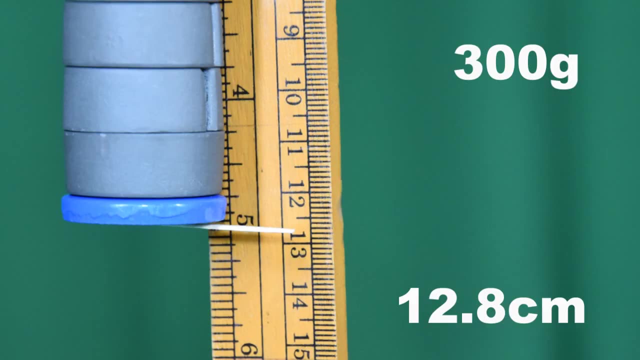 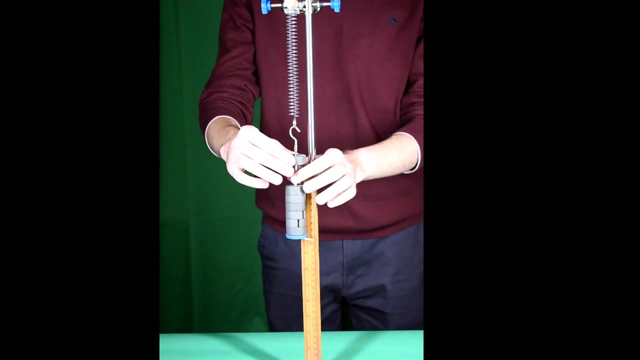 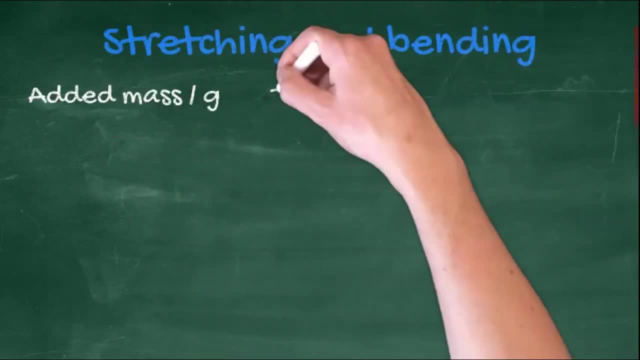 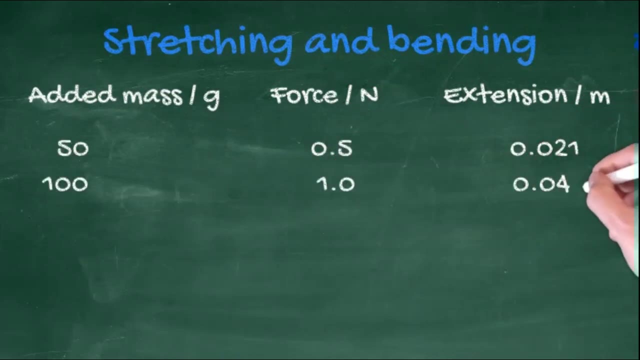 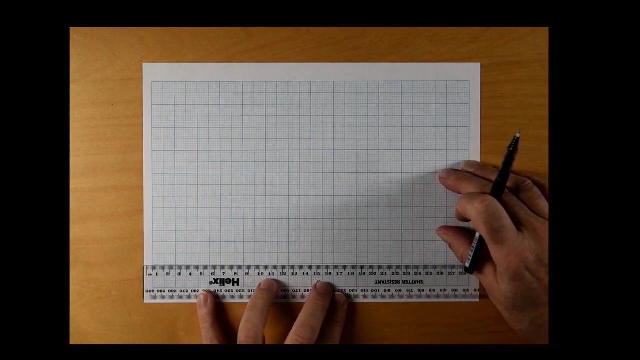 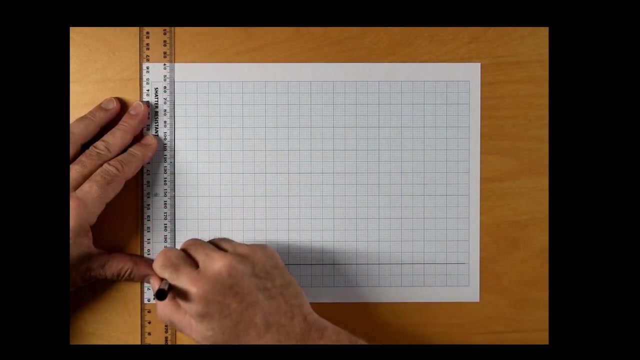 And here are the results. Grams are converted to newtons by multiplying by the value of g And, as always, here is the inevitable graph. For historical reasons to do with the original testing machines, force is always plotted up the side. 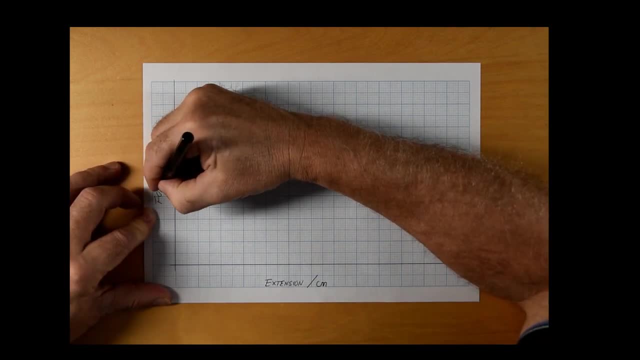 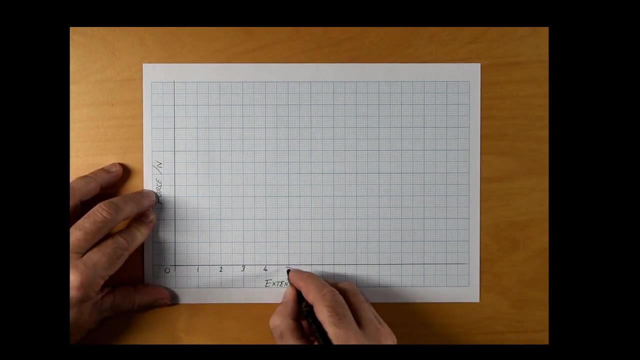 and extension. along the bottom, As you can see, the largest variable was our independent variable, but the original machines were set up to see how much force was required to stretch by a fixed amount. As always, the graph should be as big as possible with sensible axes. 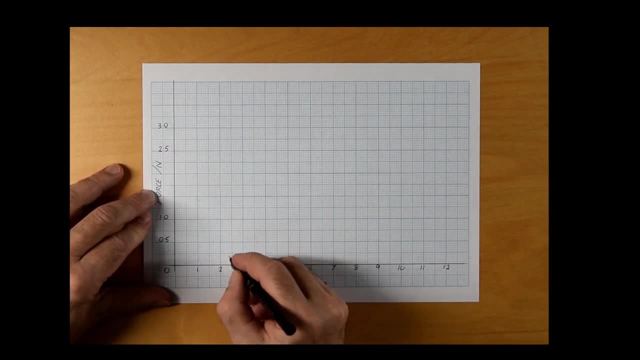 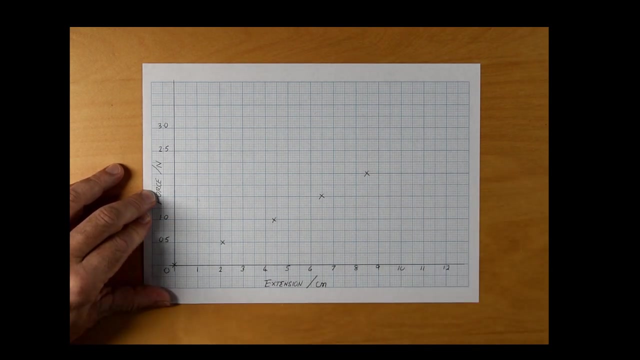 So in this case we are working in centimeters along the bottom, going from 0 to 13.. and working in Newtons up the side, going from 0 to 3.5.. 0, 0, once again, is a valid point and should be plotted. 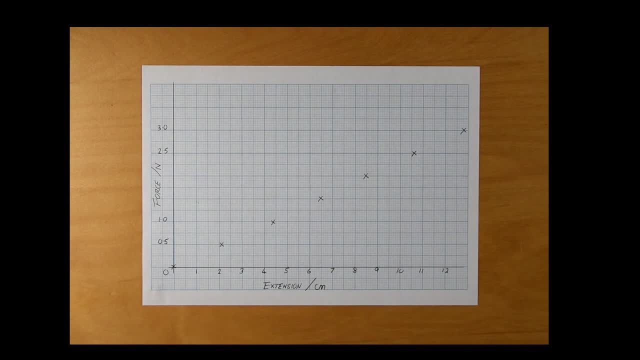 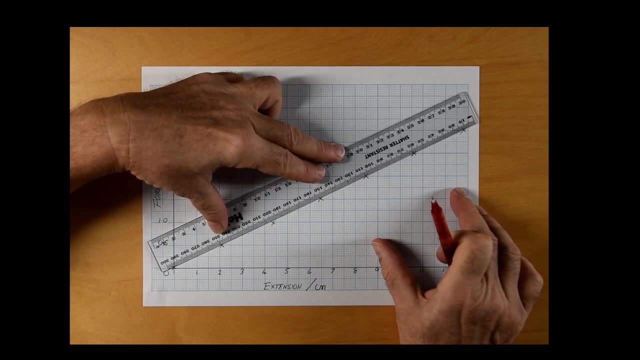 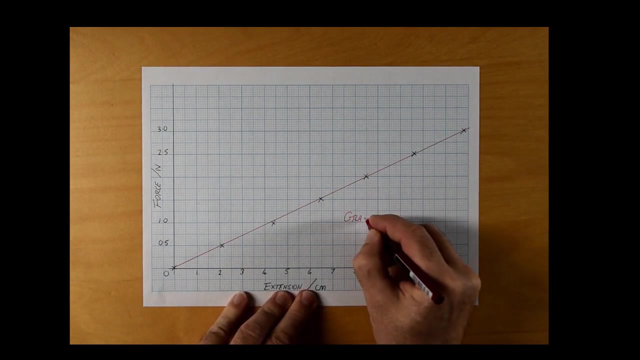 The plots clearly produce a straight line. A line of best fit should be drawn with a ruler going through 0, 0.. The gradient of this line will be force over extension or f over x. The gradient is constant for any particular spring, and this is called the spring constant k. 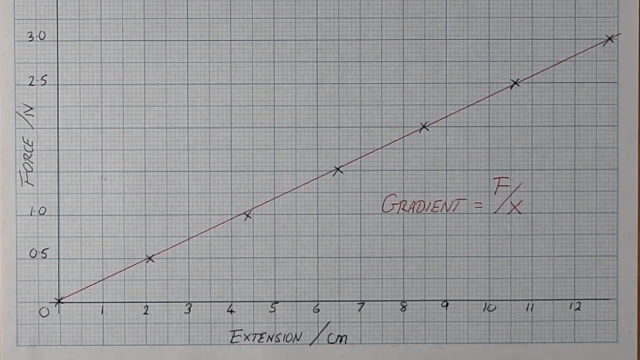 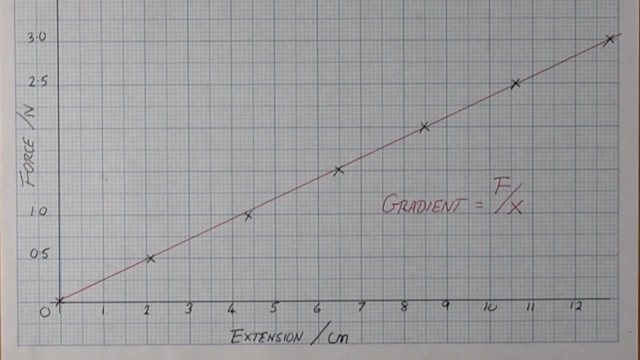 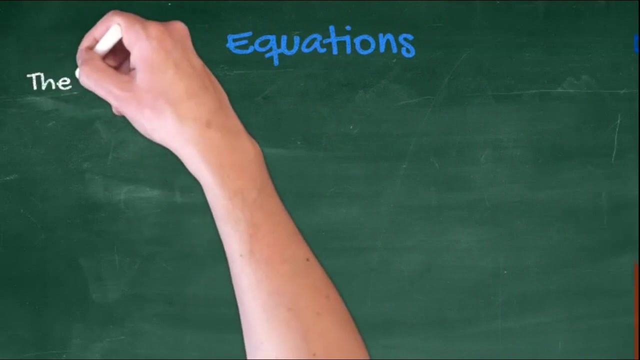 This graph produces a straight line going through the origin. It is directly proportional And this straight line shows that the relationship between the two lines is not a straight line. It is a straight line going through the origin. The relationship is linear. There are two equations that relate to this graph. 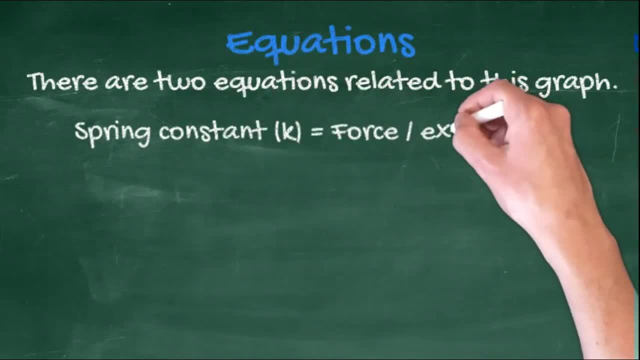 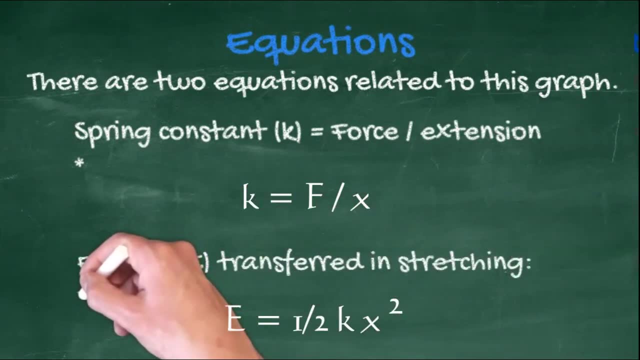 The spring constant k is equal to the force divided by the extension, or k equals f over x. The energy transferred in stretching the spring E is equal to a half kx squared. The我 NEED isn ±08k. The voltage transferred in splitting is sqaure. 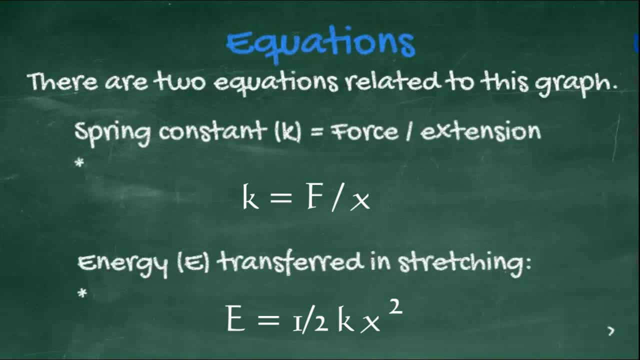 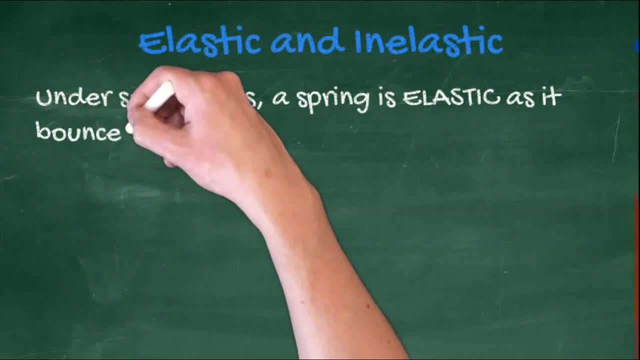 You need to know the first and be able to use the second. If the spring run is smaller than 10, should have an x squared Under small loads. a spring is elastic, Hmm, as it bouncing back to its original shape If something stretches and then remains distorted. 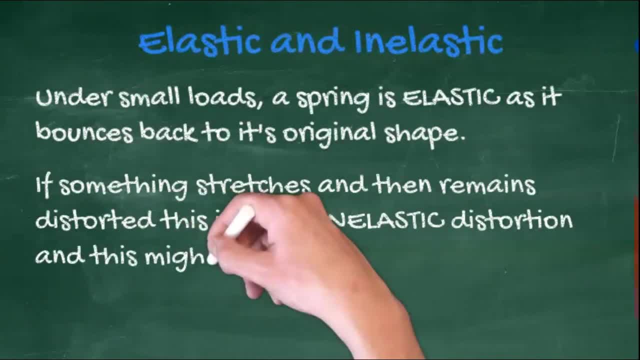 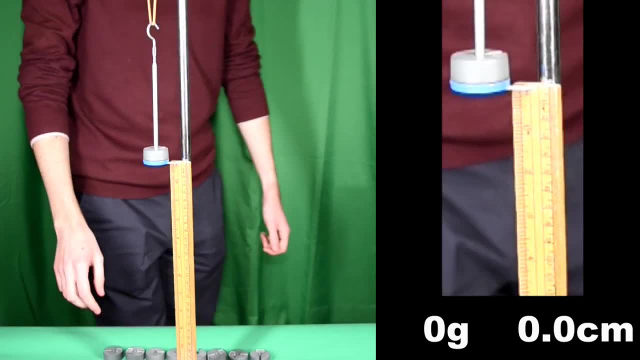 If something stretches and then remains distorted, this is called inelastic distortion. this is called inelastic distortion. an this could happen to a spring and this could happen to a spring load, for example. It turns out an elastic band isn't really elastic. And what we're going to do? 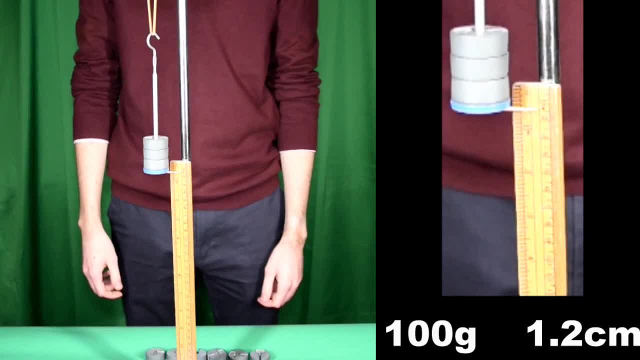 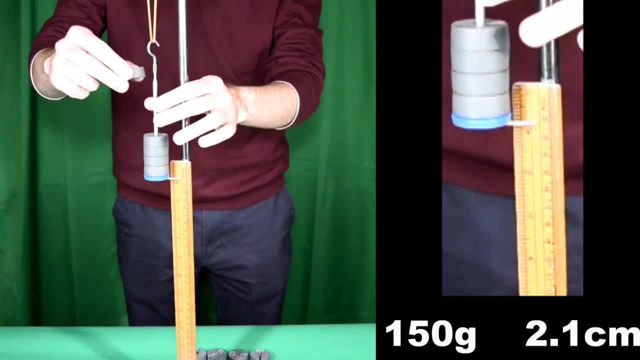 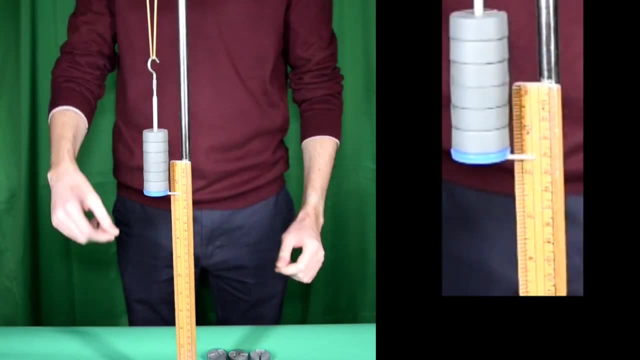 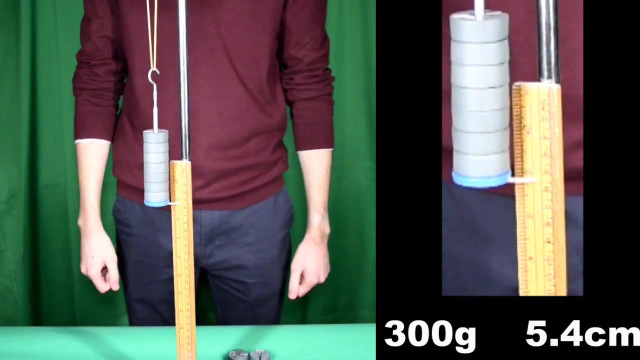 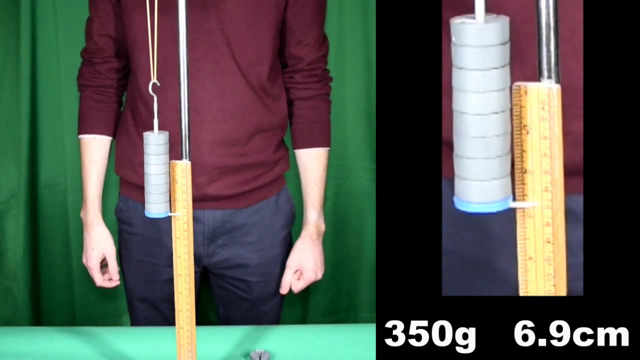 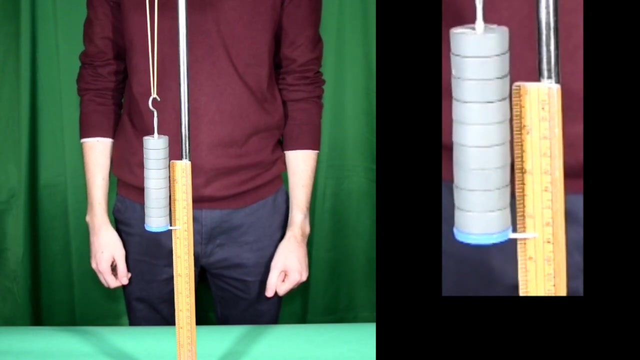 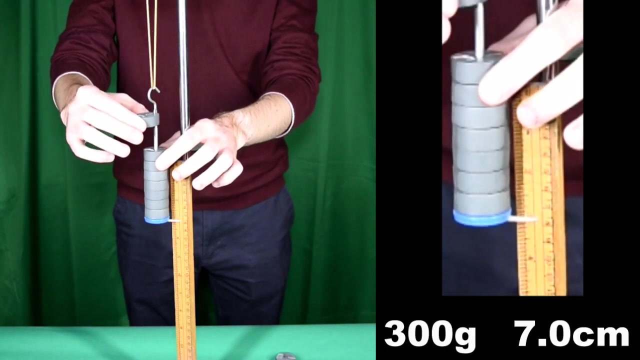 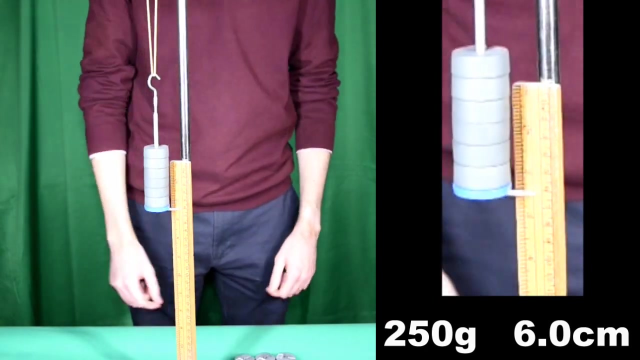 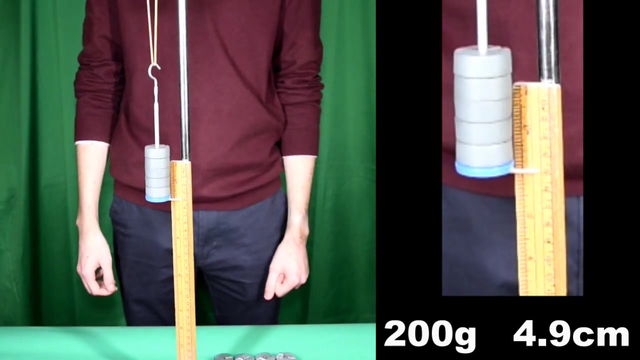 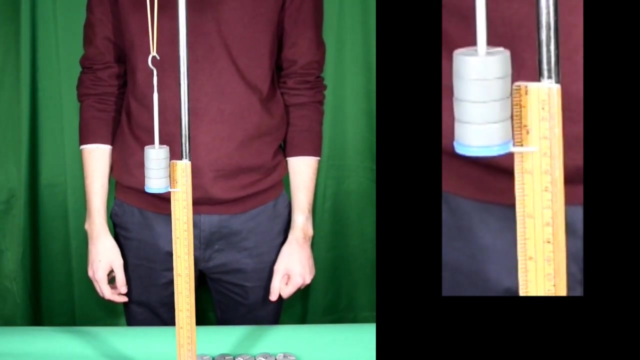 this time is: load the elastic band with 50 gram masses and try and keep the time interval between each change the same. We'll then unload them and plot a graph of the results. you at first sight, it would appear that the loading and unloading characteristics of the elastic band 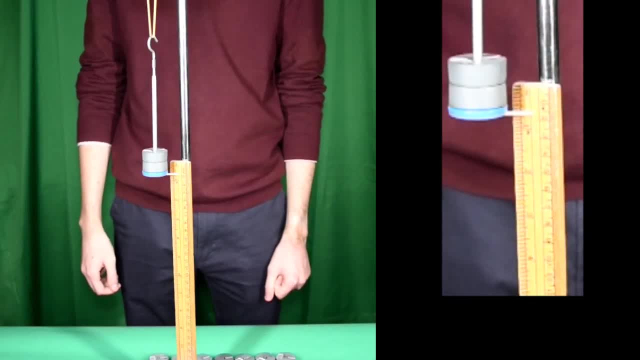 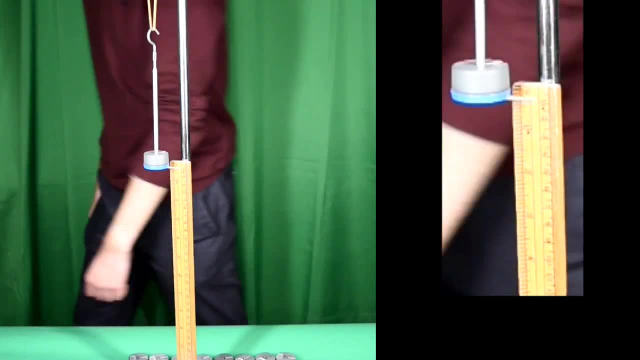 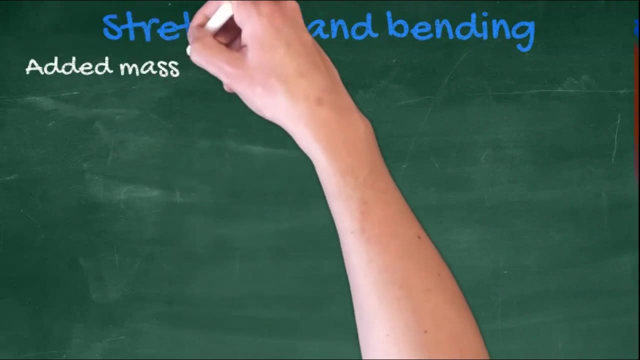 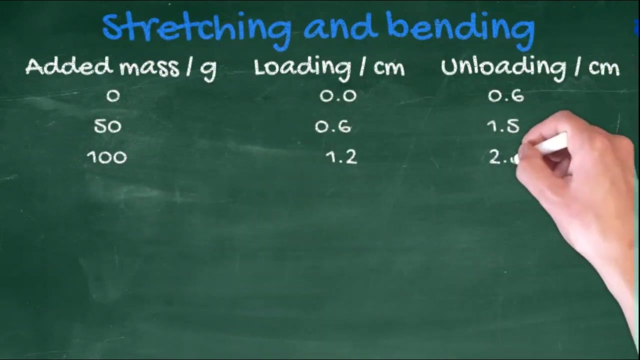 are slightly different. This is because, as you stretch an elastic band, bonds are breaking and remaking and the band gets very slightly warmer. Here are the results for the elastic band in a table. I haven't converted the grams into newtons because I'm simply going to draw this as an 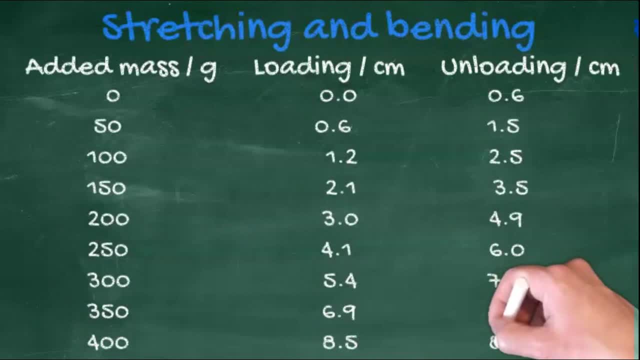 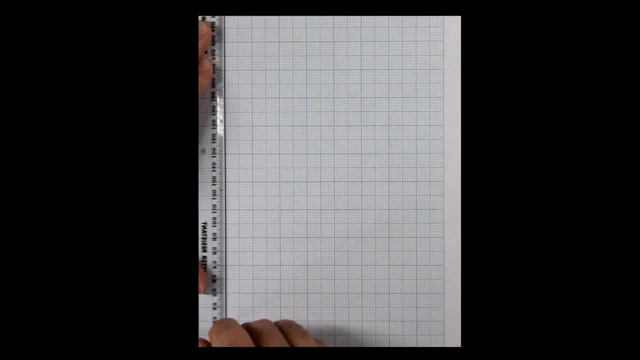 example of the graph for an elastic band And the shape won't change if I don't do the conversion. This elastic band experiment is a suggested practical. It's not in the learning outcomes, so I guess they can only ask you questions relating to the graph, for example. 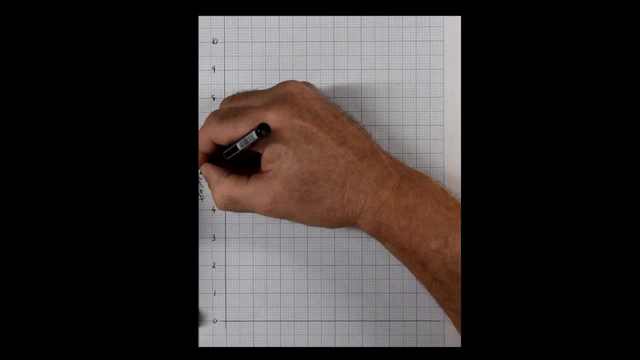 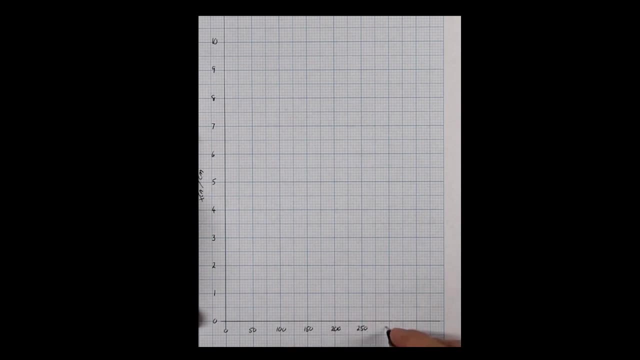 This time I'm going to put added mass along the bottom, the independent variable and the extension in centimeters up the side you. I'll plot the points for when I loaded the elastic band in black pen, you And the unloading in pen. 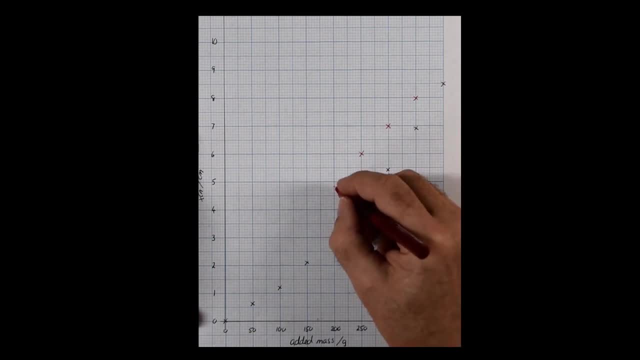 You. So this is the topic idea. All I'm going to do is simply flavours and add. we don't need to yards over that layer. I killed the half dimensional dough. A line of best fit shows a typical hysteresis curve, typical for an elastic band and this: 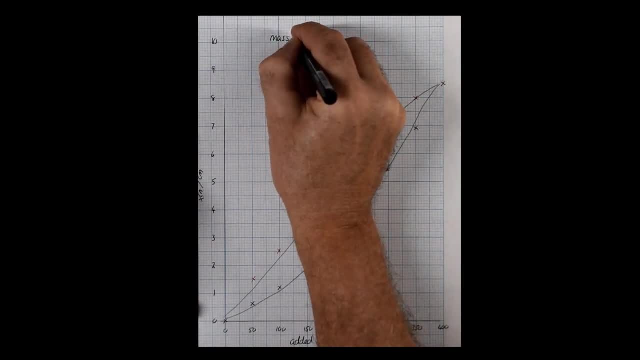 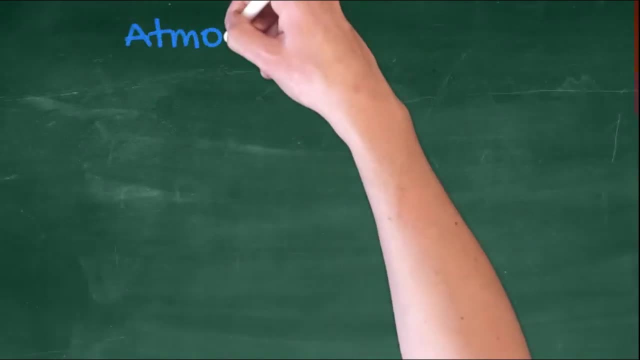 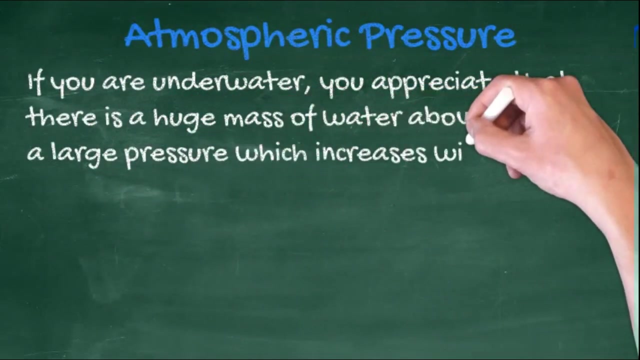 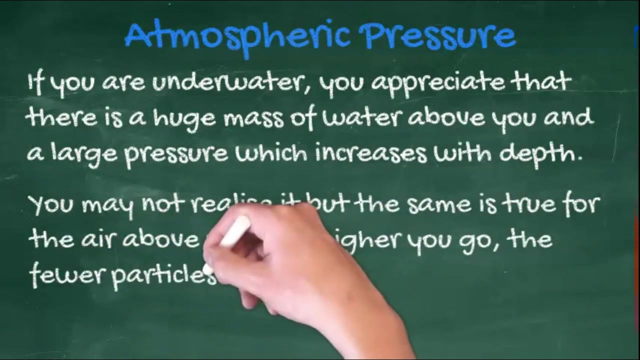 area between the two curves is the amount of energy used up in heating the band when you stretch it. If you swim underwater, you appreciate that there is a huge mass of water above you and a large pressure which increases with depth. You may not realize it, but the same thing is true for the air above you. 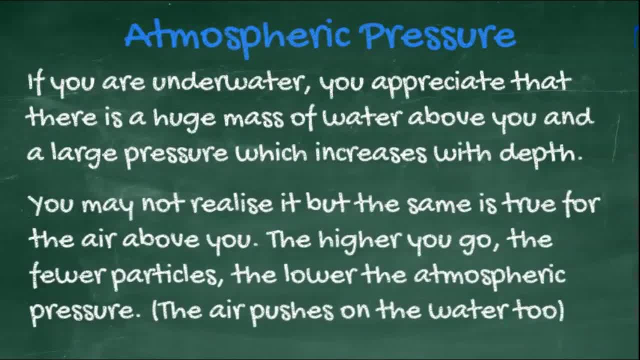 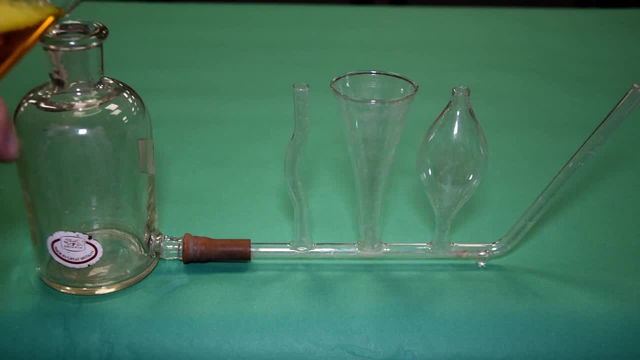 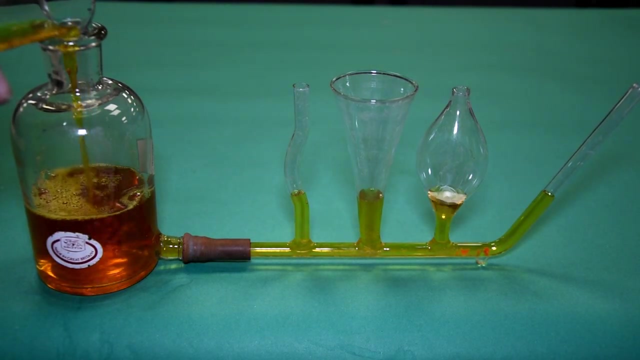 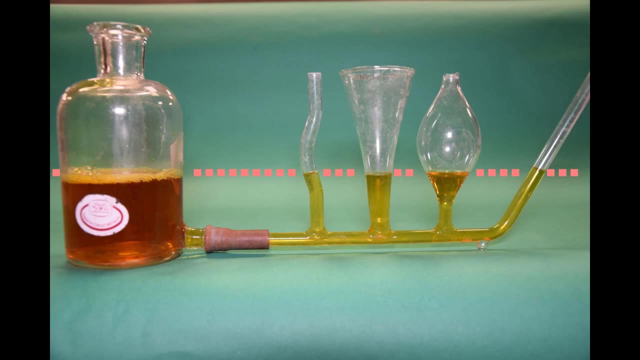 The higher you go, the fewer particles, the lower the atmospheric pressure. Now that air also pushes down on the water and as this demonstration shows, the air pressure is the same on the surface of the liquid, no matter what the shape of the container. The height of the liquid shown by the dotted line is consistent. 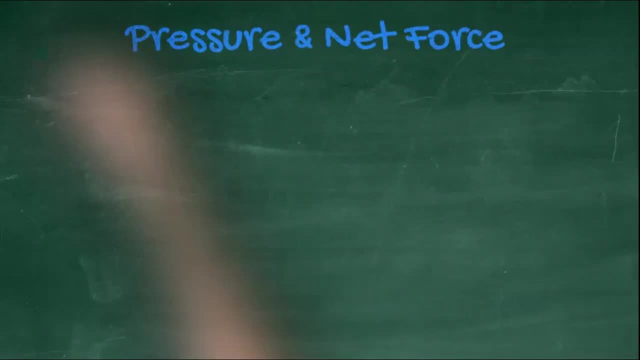 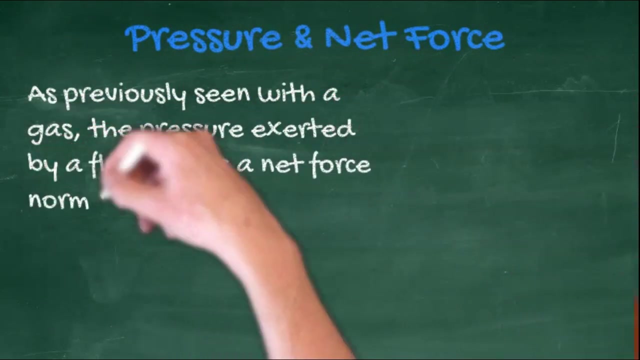 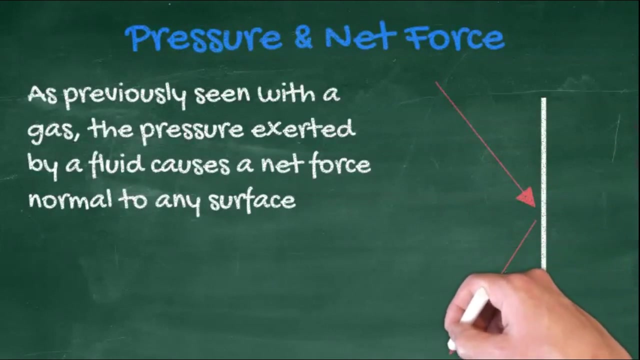 istership curve, As seen previously with the gas. the pressure exerted by the fluid on the surface of the container is same as the liquid on its surface. fluid causes a net force normal to any surface. So the liquid particles collide with the surface and rebound off. but there is a component perpendicular to 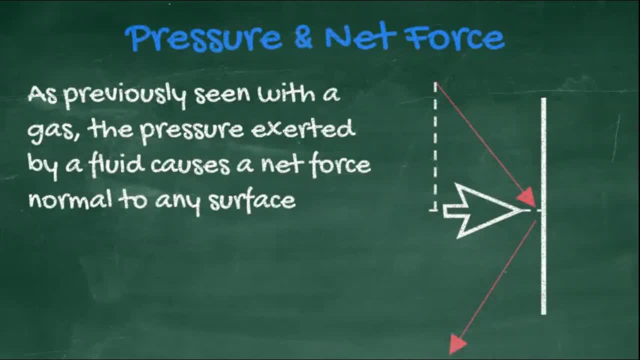 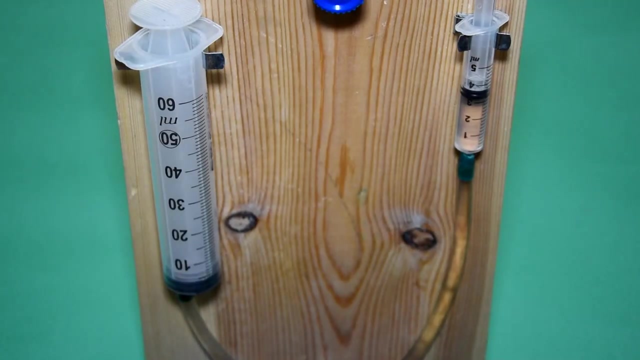 the surface of the container. The formula used to calculate pressure is: pressure equals force over area, and you are expected to know this. Finally, the units of pressure are Newtons per meter squared or Pascals. A demonstration with two different sized syringes and an incompressible fluid. 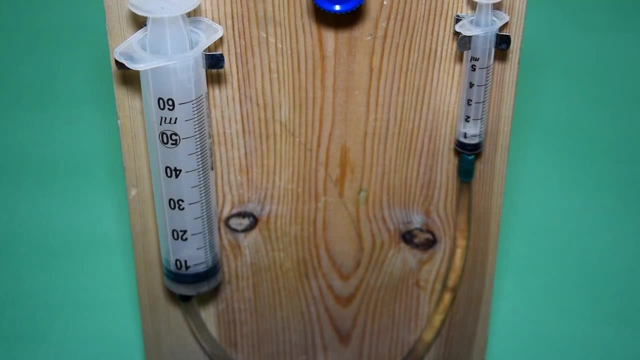 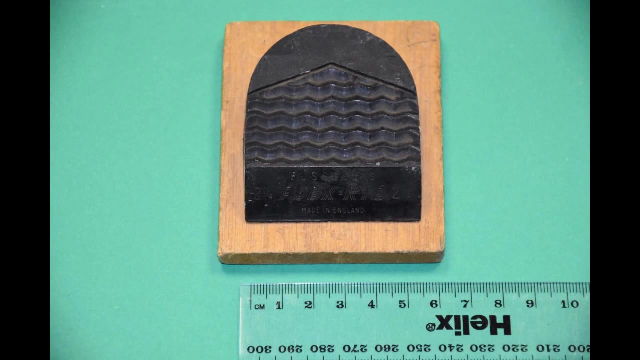 shows that the smaller surface area on the small syringe means that less force is required to move the big syringe. Rearranging the equation gives you force equals pressure times area, so the smaller area requires less force. There are numerous potential calculations from the area of the heel. 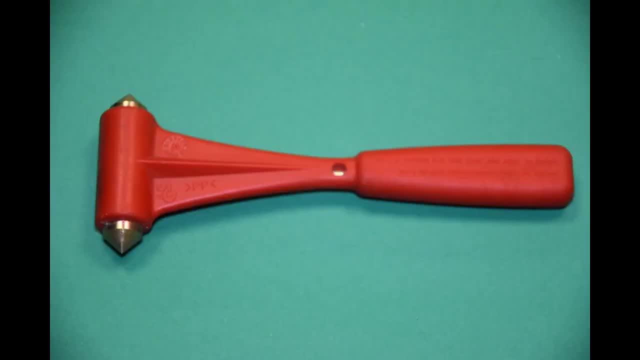 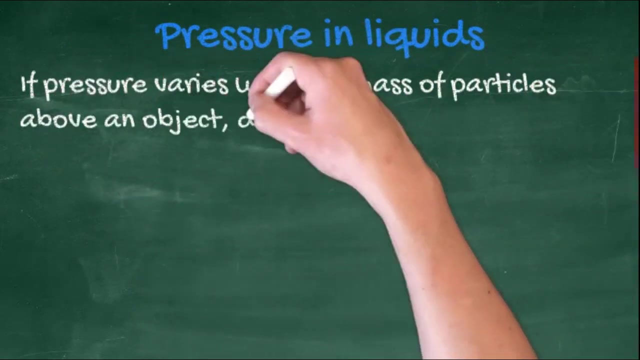 of a shoe, to having to explain why a hammer for breaking glass has a very small point, or even that a thumbtack has a narrow point. Pressure in liquids. If pressure varies with the mass of particles above an object, density must be a factor. 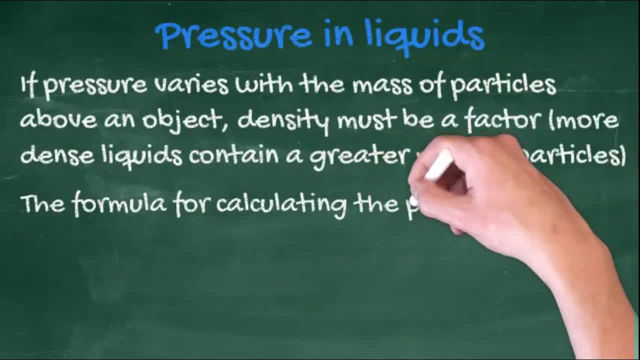 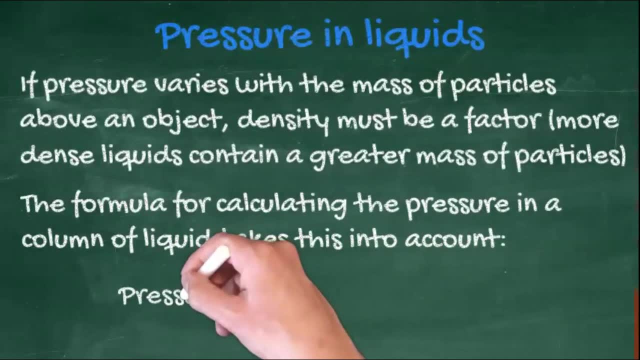 More dense liquids contain a greater mass of particles in the same volume. The formula for calculating the pressure in a column of liquid takes this into account. The pressure in a column of liquid is equal to the height times the density times gravitational field strength. This demonstration shows simply: 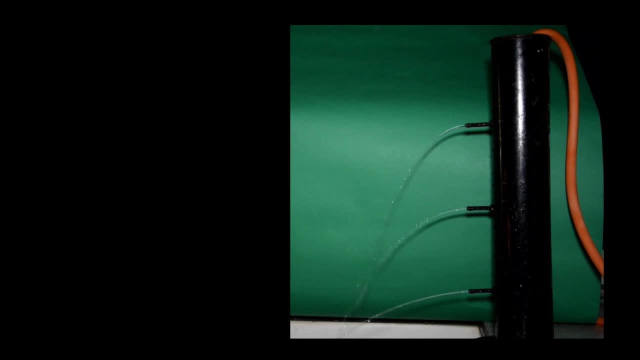 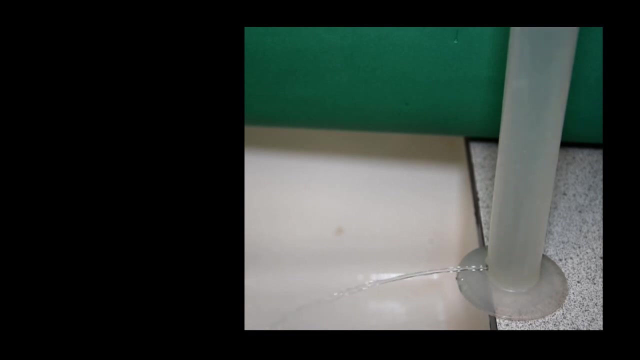 how the pressure changes with height of liquid. the jet at the top doesn't go as far as the jet at the bottom because it has less height of liquid above it. And a second demonstration where you can see that, as the height of liquid in the 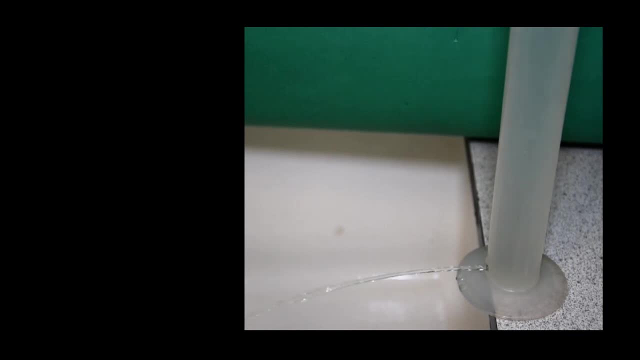 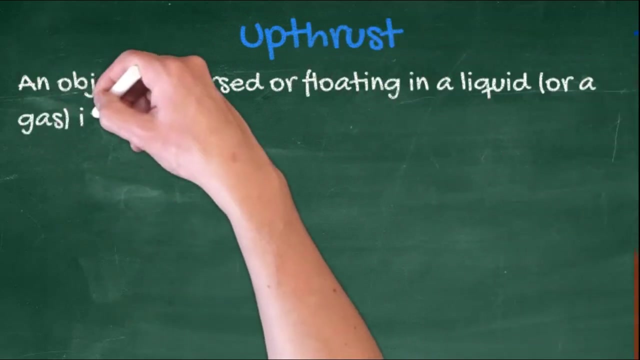 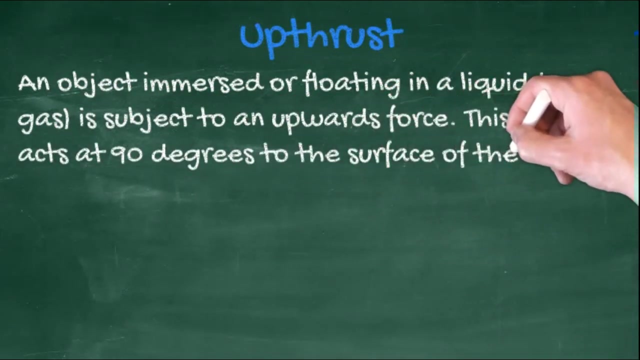 measuring cylinder increases the distance the jet travels increases as well. As the liquid goes down in the measuring cylinder, the pressure reduces and the jet coming out of the bottom doesn't travel as far Does an object float? An object immersed or floating in a liquid or a gas is subject to an upwards. 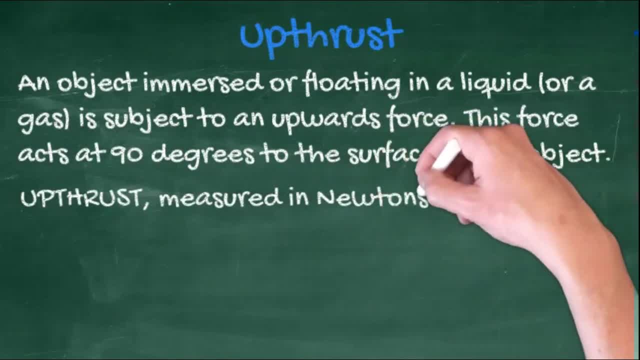 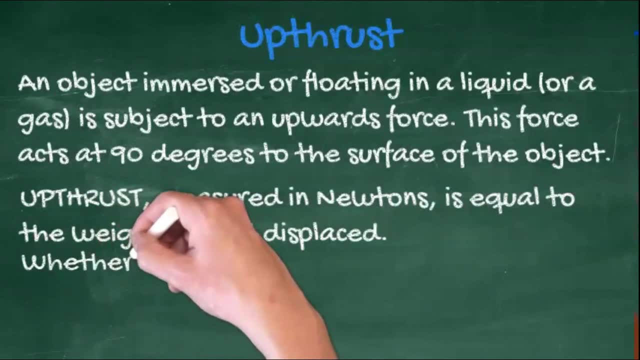 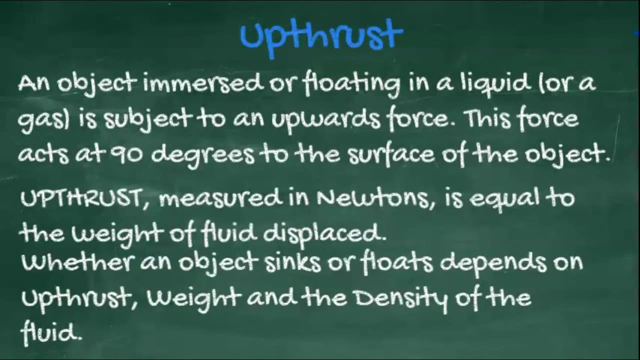 force. this is called up thrust. this force acts at 90 degrees to the surface of the object. Up thrust measured in Newtons is equal to the weight of the fluid displaced. Whether an object sinks or floats depends on up thrust and the weight and the density of the fluid. 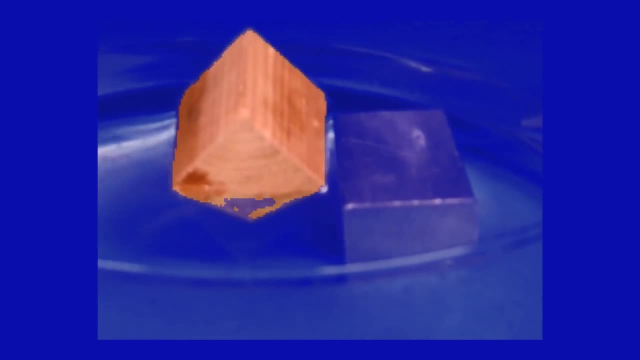 The wood floats because the mass of the wood that's in the water is less than the mass of the water displaced. If you like, it should be weight. The aluminium block, on the other hand, sinks because the weight of the block is much greater than the weight of the water displaced. 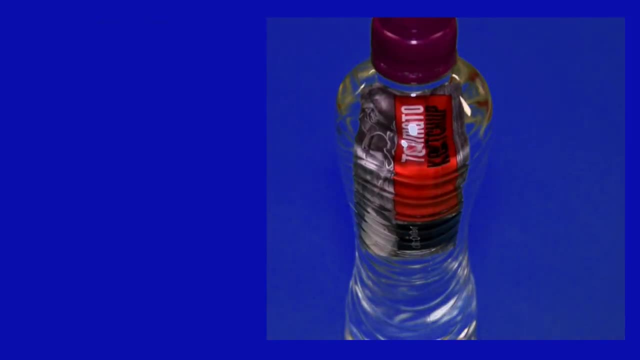 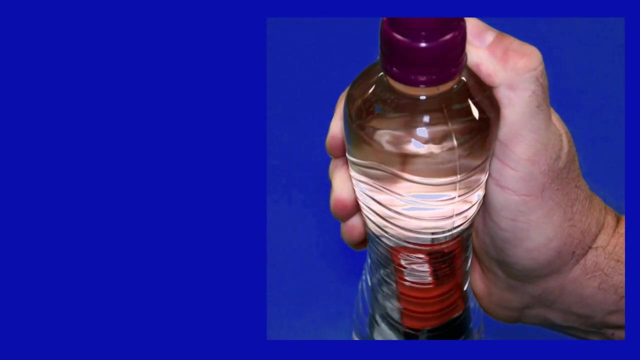 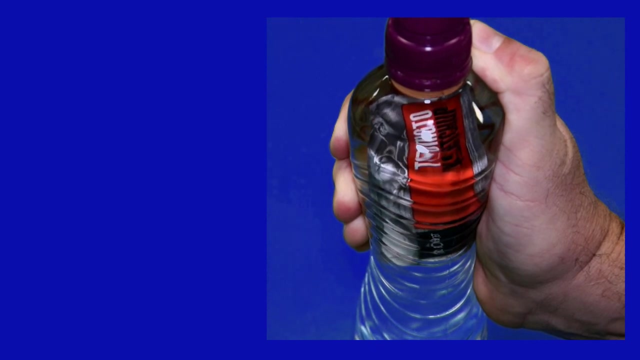 A sachet of tomato ketchup has almost exactly the same density of water, but there's a little bit of air. If you squeeze the container, water is incompressible, so the air inside the sachet squeezes, the density increases and the sachet falls down When you stop squeezing the container. 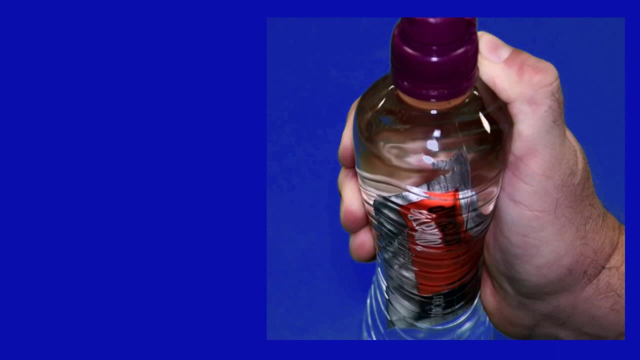 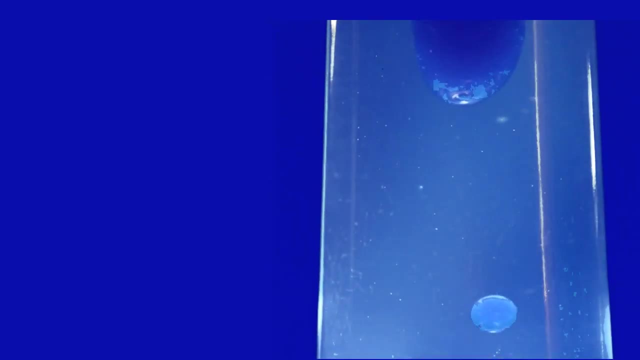 the density is slightly less than water and the sachet comes up again. This is often called the Cartesian Diver. A lava lamp basically consists of wax in water. Now, they have very similar densities, but when the wax is heated it spreads out just a little bit. the particles open up, and because it therefore has